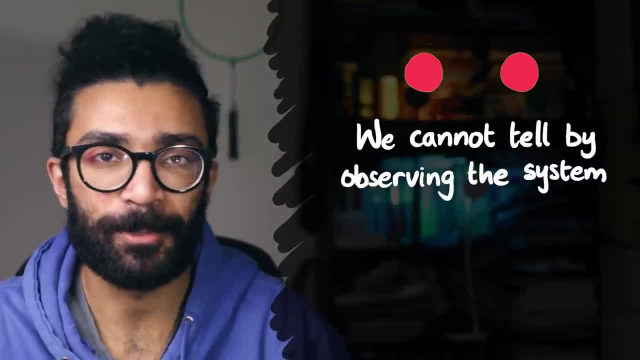 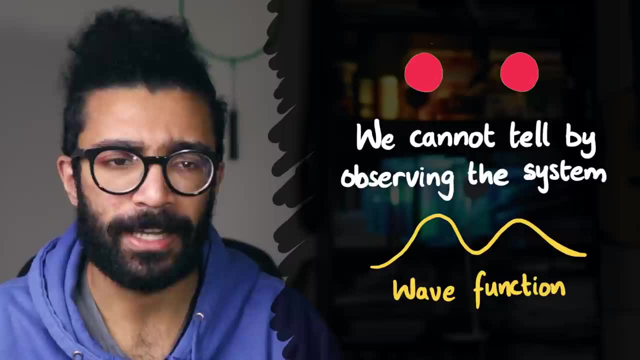 of these bosons. We can understand the impact that this indistinguishability has by considering the wave function of any system we happen to be studying Now. a wave function can basically be thought of as a mathematical function that contains all of the information that we know about our system. For example, if our system consists 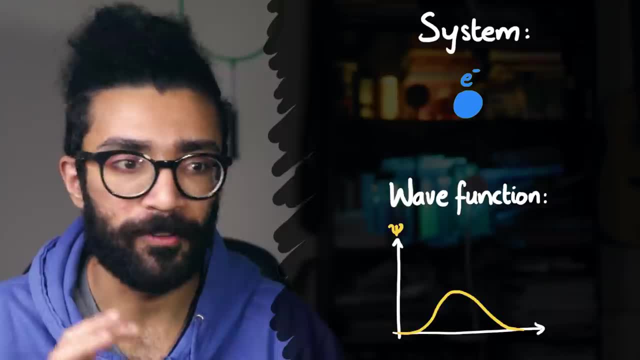 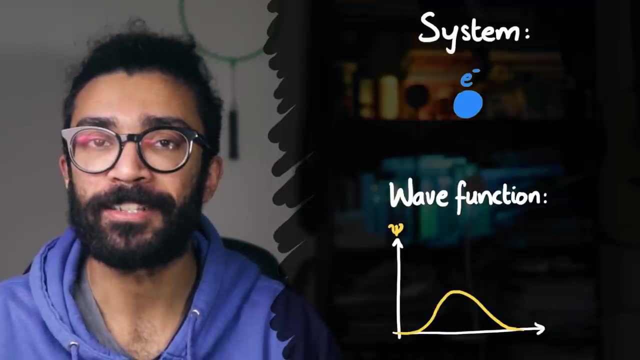 of just a single electron, then from the wave function of our system we can calculate the probability of finding that electron at different points in space. Specifically, it turns out that if we square any wave function, technically we take it square modulus, then that is directly. 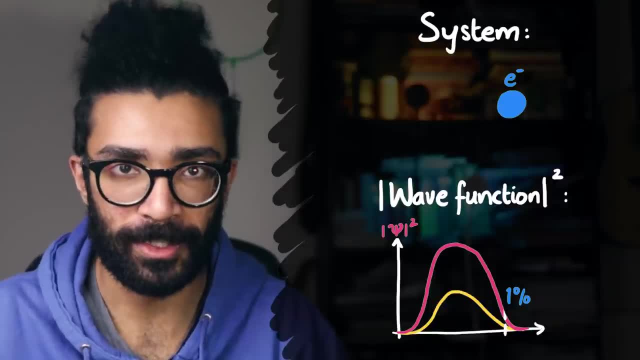 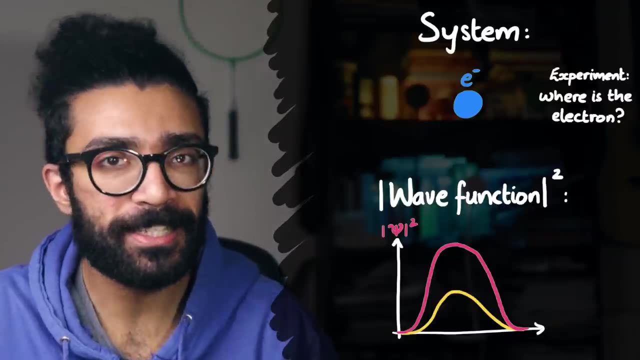 related to the probability of certain experimental results occurring when we make a measurement on our system, when we conduct an experiment on it. I've also made many videos discussing this idea in a bit more detail, so please do check out my quantum mechanics playlist for more. 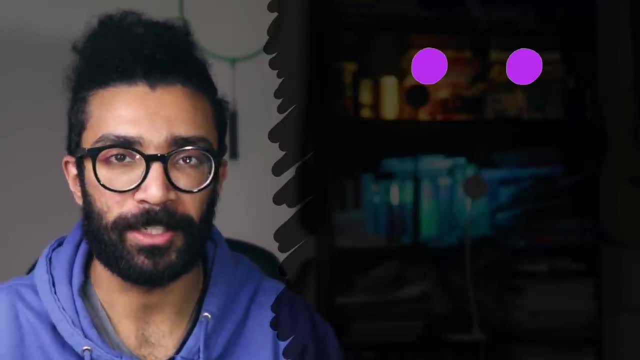 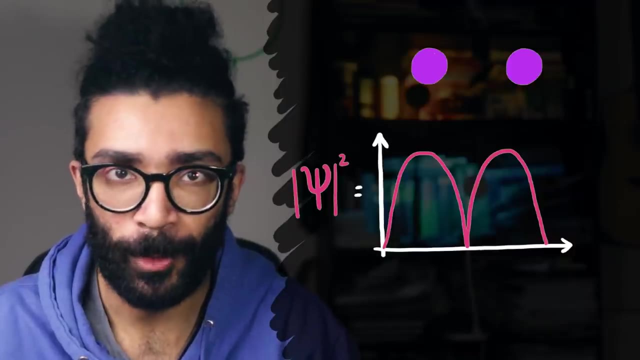 But if we now consider two indistinguishable particles- we can't tell these particles apart- and we take this system's wave function and we square it, then this wave function, squared, must behave in such a way that it's identical whether our two particles are found in this. 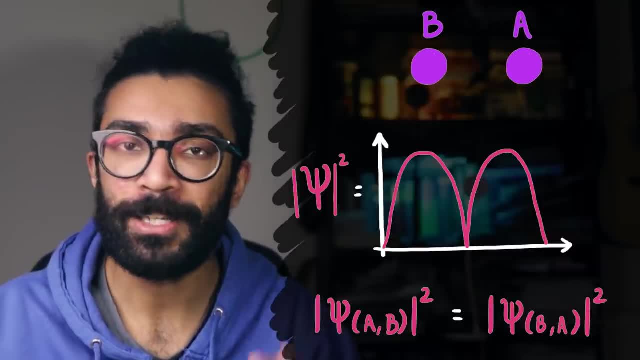 orientation or in this orientation. So if we take this wave function squared and we square it, then this wave function squared must behave in such a way that it's identical whether our two particles are found in this orientation or in this orientation. In other words, if we swap particles A and B, the wave function squared should look exactly. the same, because we shouldn't have any way of knowing which particle is which, Whereas if the wave function changed when we swapped these particles, then we would be able to tell. there would be some experiment that we could do on our system that would tell. 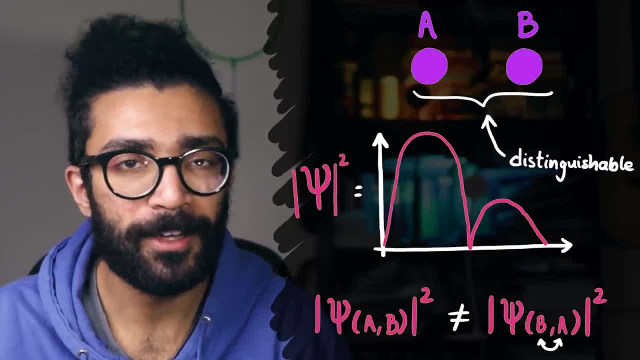 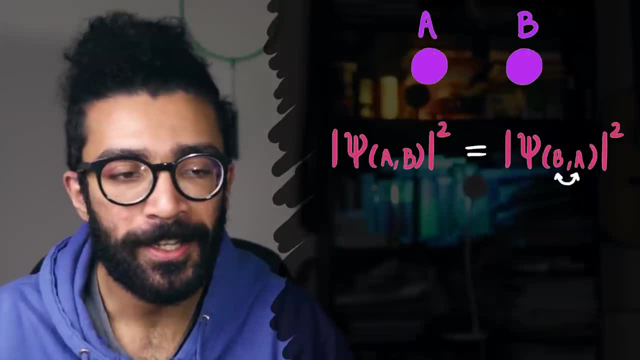 us which wave function squared we had for that particular system and therefore which orientation we had our particles. So basically, the square of the wave function when we've got the orientation must be the same as the square of the wave function when we've got the orientation. 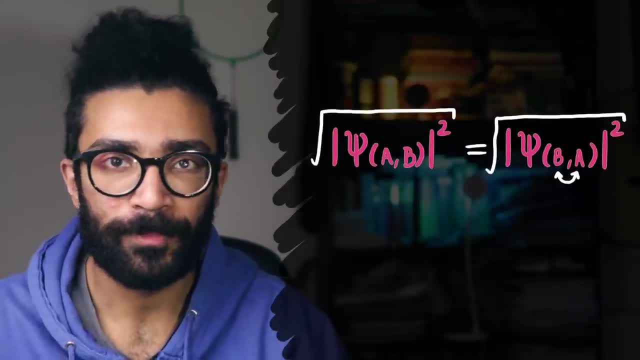 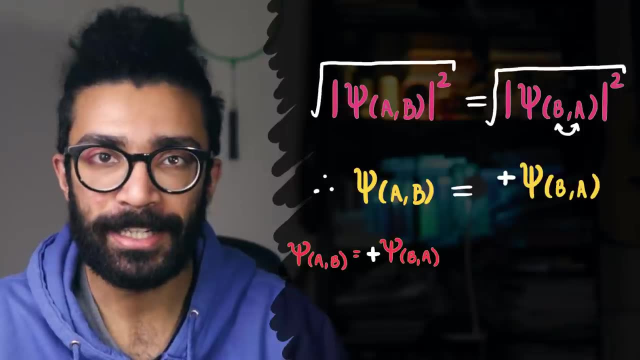 If we then take the square root of this mathematical expression, then what we find is that the wave function itself- for when we've got the particles in the orientation- must either be exactly equal to the wave function of the orientation, or it must be equal to minus the wave function. 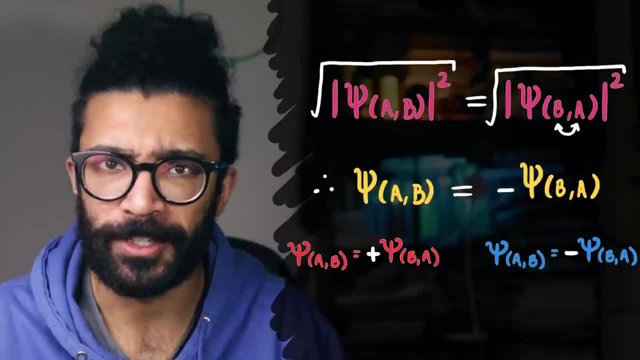 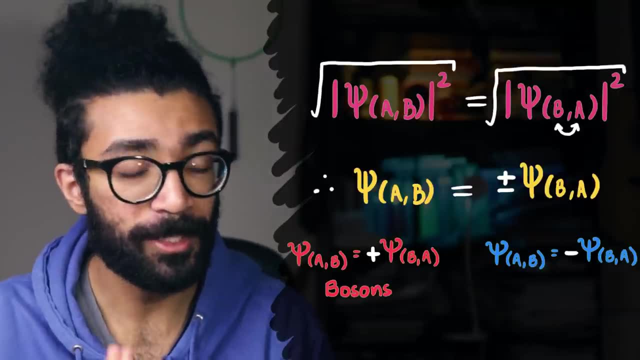 of the orientation, And so what we've done here is discovered the wave functions for two different classes of particle. The particles for which the wave function behaves are known as bosons, and the particles for which the wave function behaves like this are known as fermions. 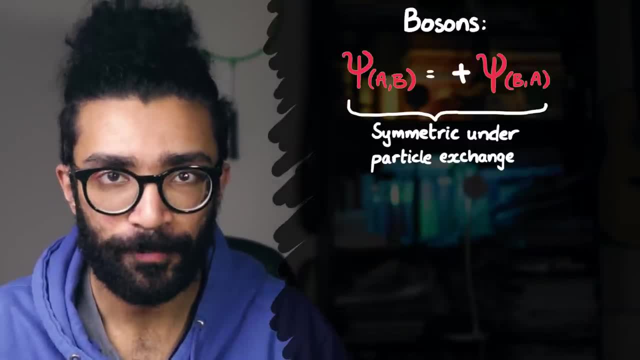 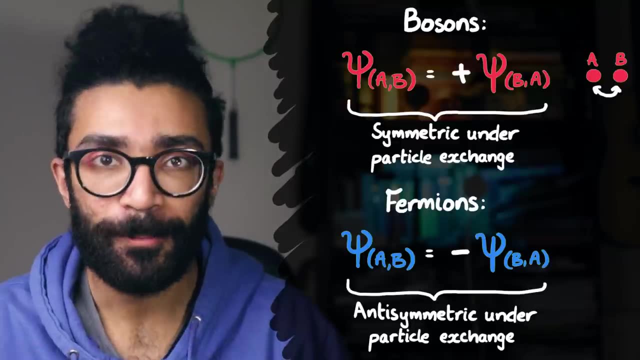 With a boson wave function, we basically say that it is symmetric under particle exchange. What this means is that the wave function is identical when we swap particles, Whereas with fermions we say that the wave function is anti-symmetric. Basically means that when 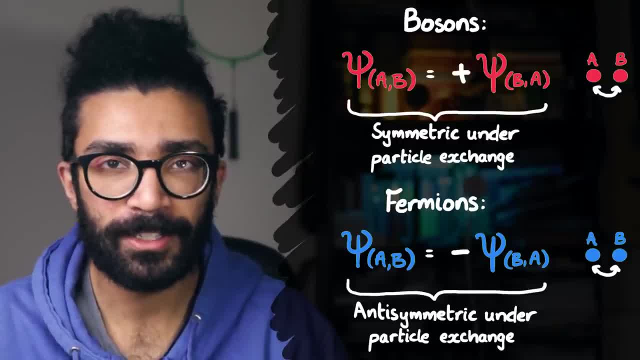 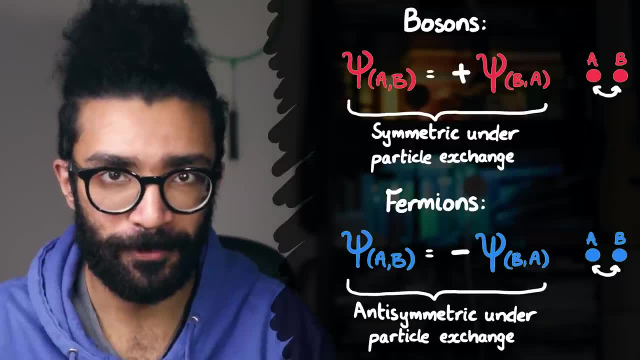 we swap the particles, the wave function becomes negative. The fact of the matter is that a symmetric wave function behaves differently to an anti-symmetric one. This is the crux of the difference between bosons and fermions, and we'll be focusing. 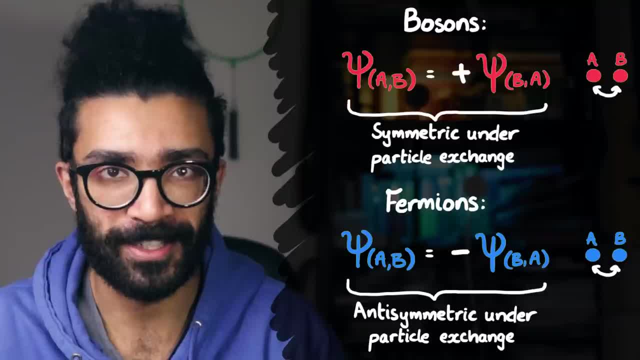 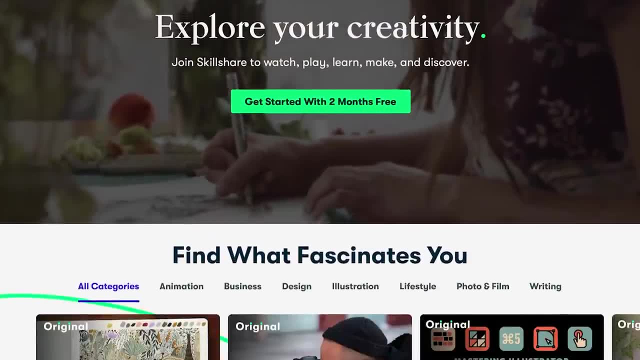 in on the behaviour of bosons in order to understand the Bose-Einstein condensate. Now, before we go any further, I'd like to thank this video's sponsor, Skillshare. Skillshare is an online learning community where you can find a large number of inspiring 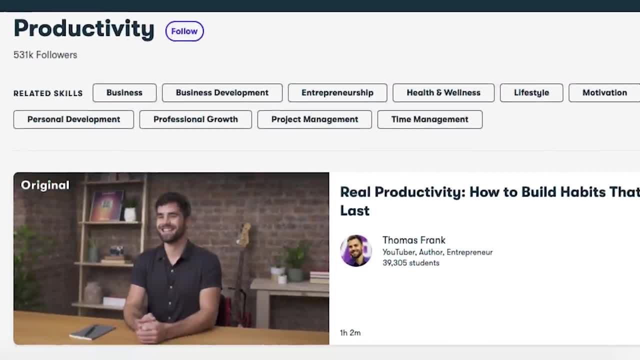 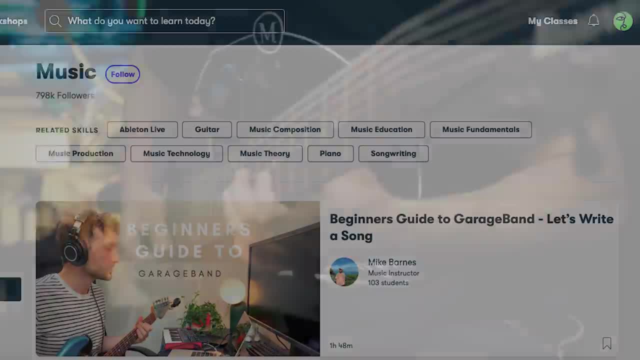 classes focusing on topics such as productivity and lifestyle, to building a business, to learning creative skills. Many of you may know that one of my hobbies is creating music. Check out my music channel linked below. Skillshare has a large number of classes on Skillshare that have taught me some really. 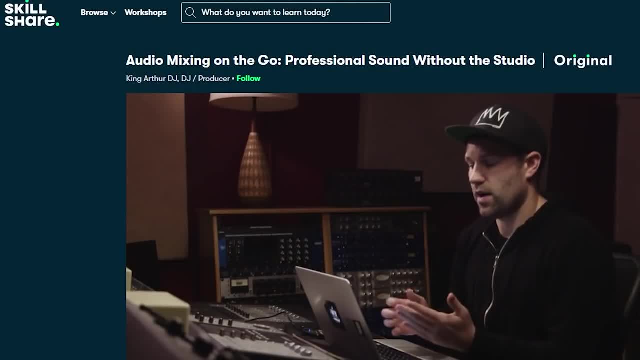 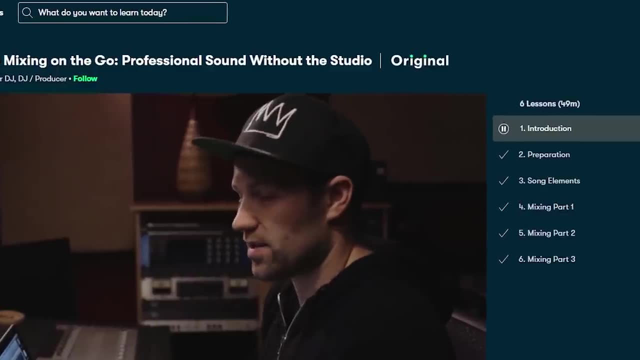 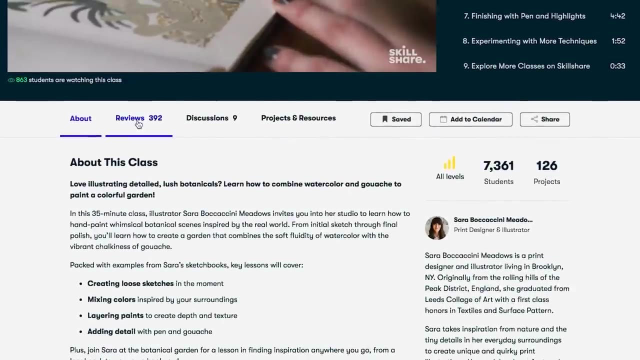 cool skills. For example, I took a class called Audio Mixing on the Go Professional Sound Without the Studio by King Arthur, which gave me lots of tips for improving my mixes without lots of fancy equipment. Skillshare has a large number of classes to choose from and it's all about learning. 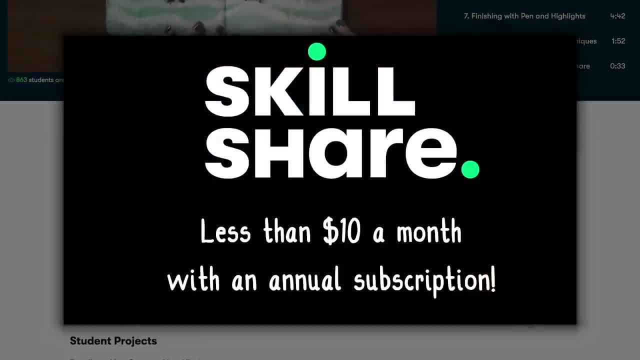 so there are no adverts And Skillshare costs less than $10 a month with an annual subscription. But the first 1,000 of you to click the first link in the description box below will be able to get a free subscription to Skillshare. 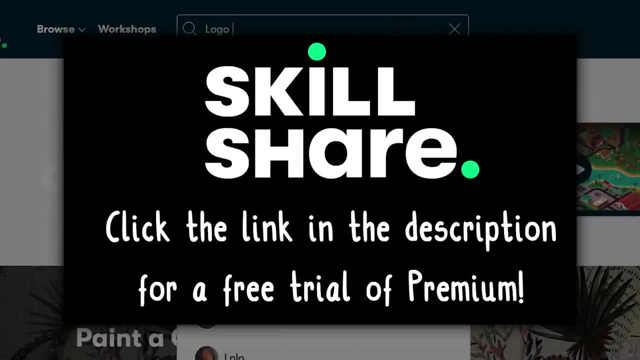 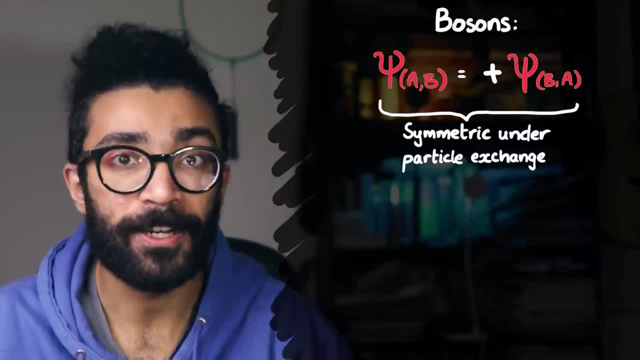 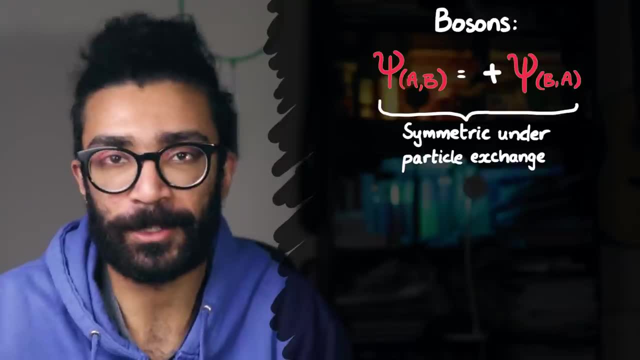 Now just to recap. we saw earlier that bosons have a symmetric wave function and fermions have an anti-symmetric wave function. To understand how we can go from this mathematical condition to the Bose-Einstein condensate behavior, we'll be looking at a rather oversimplified 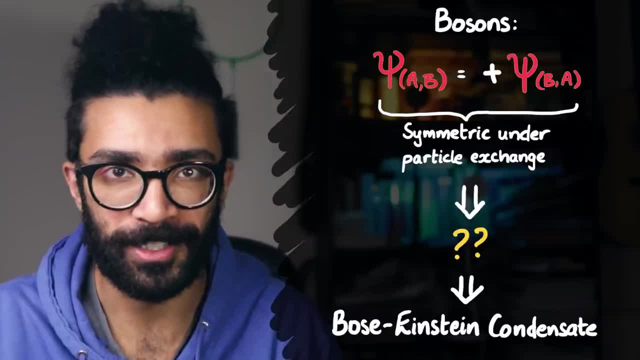 description of what's going on, but hopefully we can convey the idea appropriately. Let's now imagine that the two particles we're considering are two bosons. We'll be looking at a rather oversimplified description of what's going on, but hopefully we can. 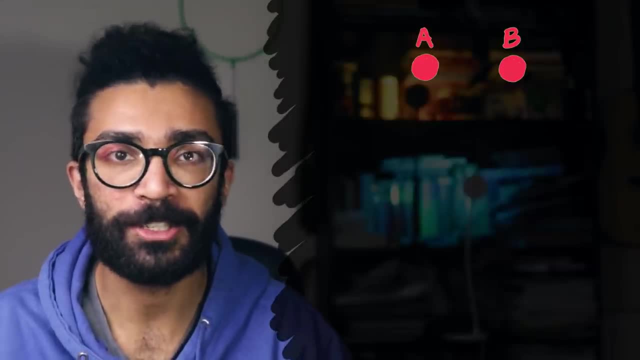 convey the idea appropriately. Let's now imagine that the two particles we're considering are two bosons, and that's why we'll be looking at a rather oversimplified description of what's going on, but hopefully we can convey the idea properly. Let's now imagine that the two particles we're considering are two bosons and they 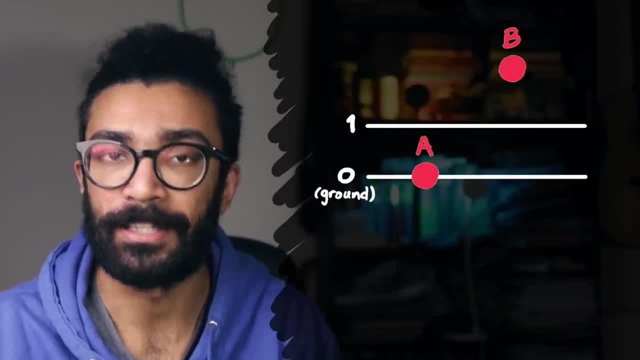 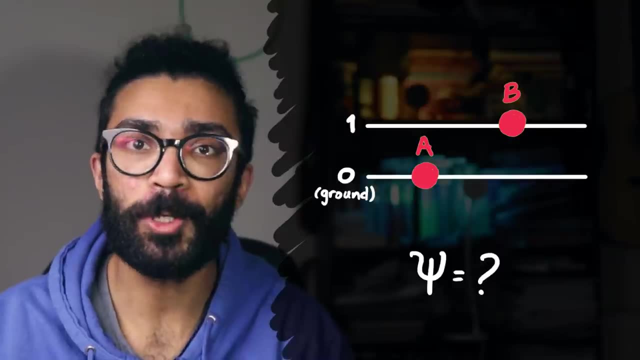 can occupy two different energy levels. The energy level labeled 0 is the ground state energy level and the energy level labeled 1 is a slightly higher energy level. If this is our system, we can work out what a possible wave function would look like for. 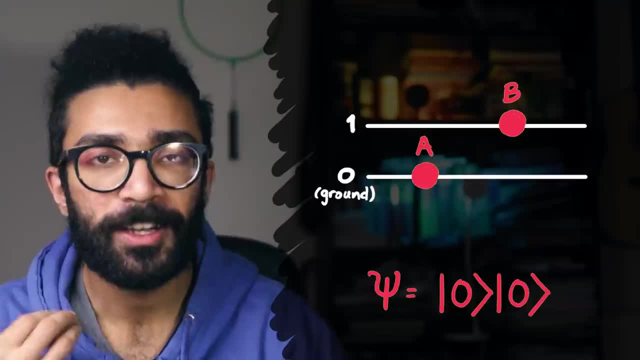 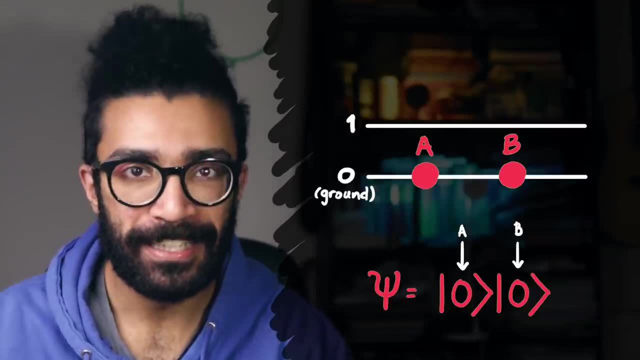 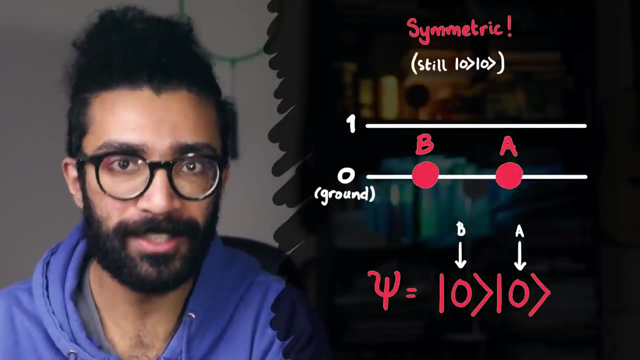 our system. It could, for example, look like this: What this represents is particle a in energy level 0 and particle b in energy level 0. This is indeed a symmetric wave function when we swap the particles, because the wave function exactly the same under particle exchange. and what this actually means is that if our two particles 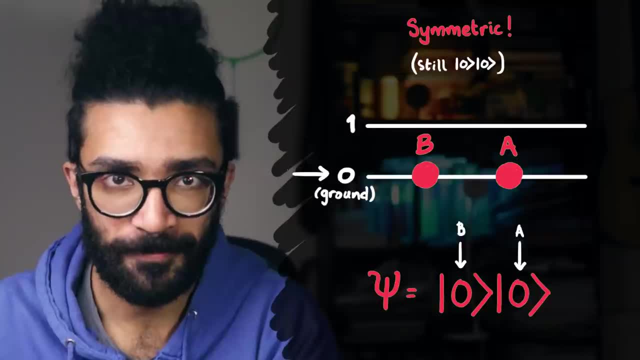 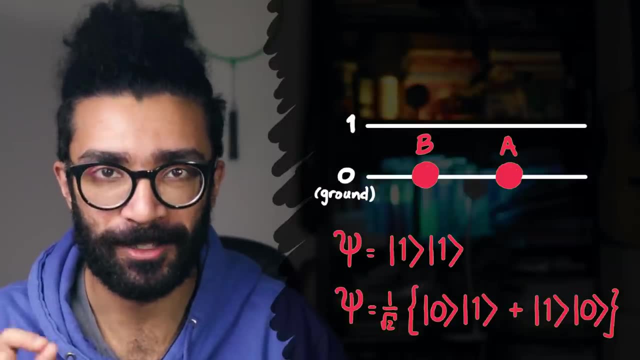 are indeed bosons. they can occupy the same state As it turns out for this particular system. there are also two other wave functions that we could construct. They look like this, but we will take a look at those in a moment. Instead, let's consider what would happen if our two particles were. 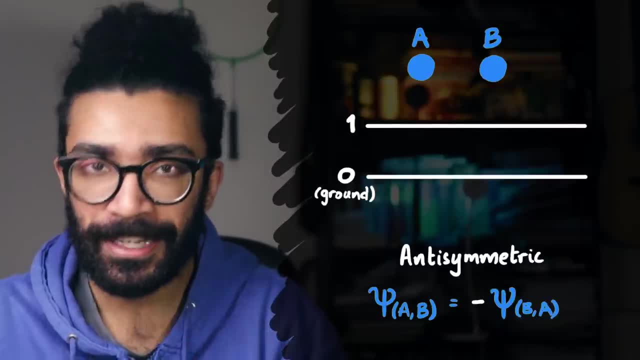 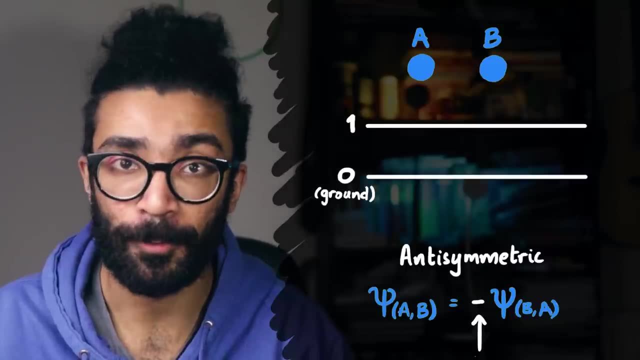 fermions, not bosons, If the wave functions had to be anti-symmetric. Remember, the condition here is that when we swap the particles, the wave function must become negative of what it used to be, and for this particular kind of system, that wave function ends up looking like this: What we've got represented. 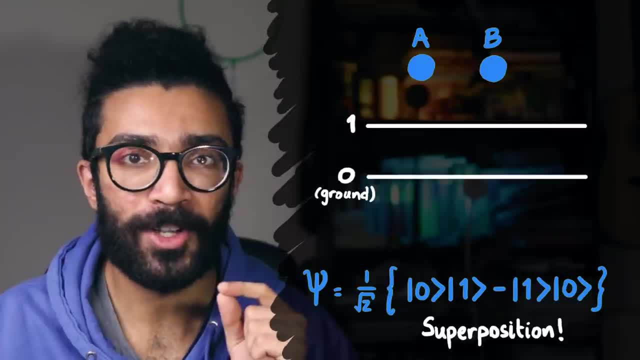 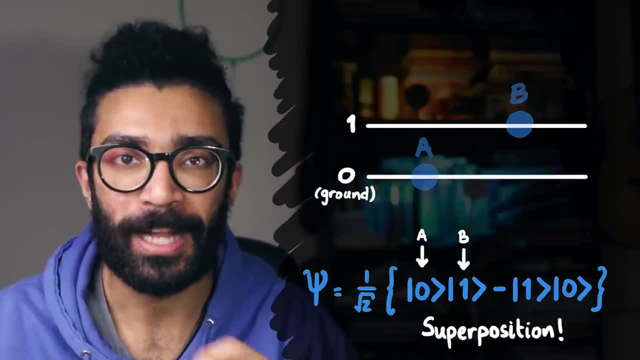 here is a superposition between the state where particle a is in the energy level zero and particle b is in the energy level one, and the other state, which is when particle a is in energy level one and particle b is in energy level zero. Now, superposition is an important idea in quantum. 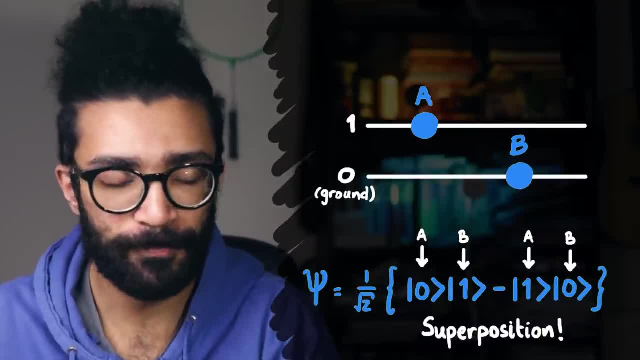 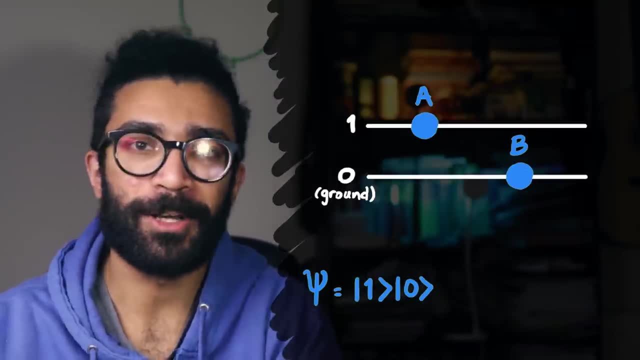 mechanics, It's when a system can supposedly occupy multiple states before we've actually made a measurement on it, and when we do make a measurement, the system will collapse into one of those states. Again, more discussion on this in my quantum mechanics playlist Now. the reason that our fermionic wave function looks like this is 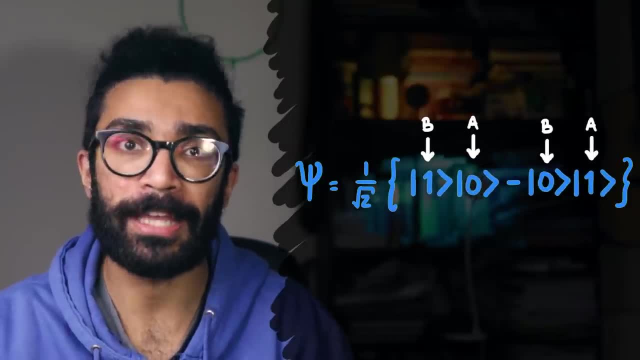 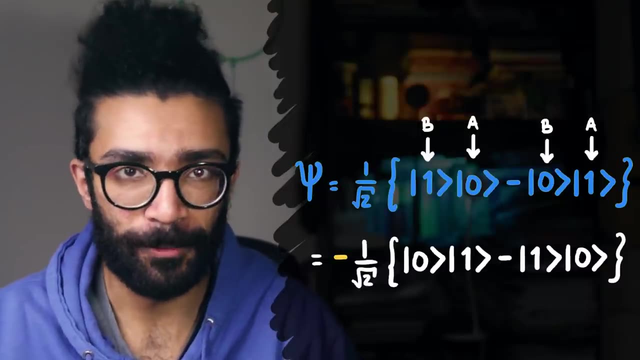 because if we swap the two particles now, if we label particle a as b and b as a, then we see that the wave function becomes negative of what it used to be, Which is exactly what we need for fermions. we need an anti-symmetric wave function, But interestingly it's not actually the superposition. 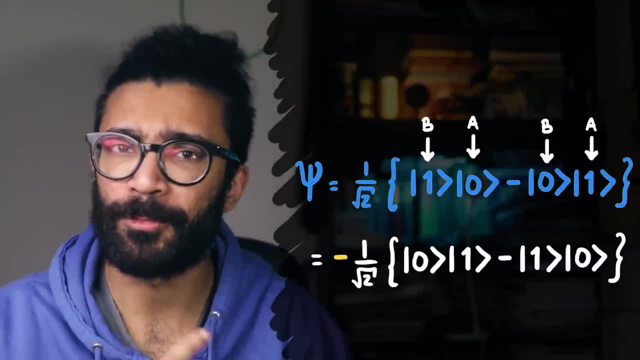 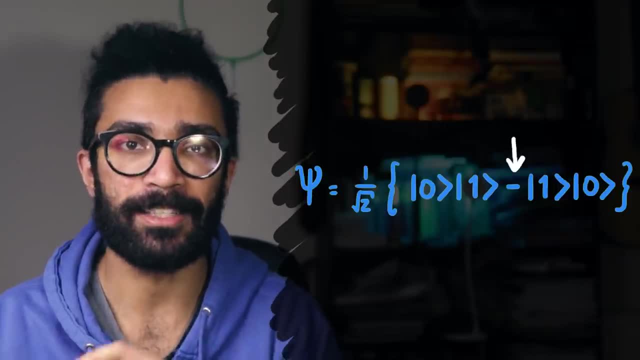 that makes our wave function anti-symmetric. We need an anti-symmetric wave function. As we can see from one of the bosonic states we've also got a superposition, But in the fermion wave function it's the negative sign. here specifically that makes it an anti-symmetric wave function. 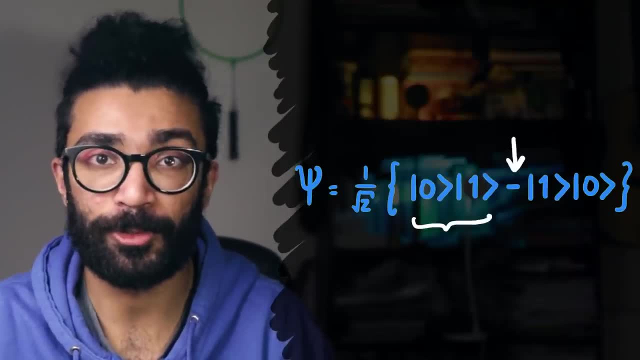 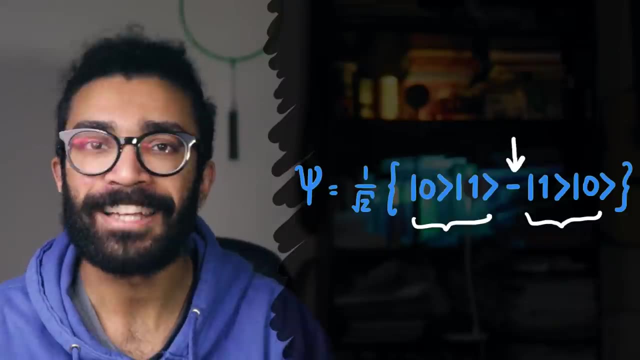 Now, this negative sign has got something to do with the phase between the two possible superposed states, but it's not really relevant to us here. The important thing is that when we swap the particles, the wave function becomes negative And, as we've already mentioned, this is what we 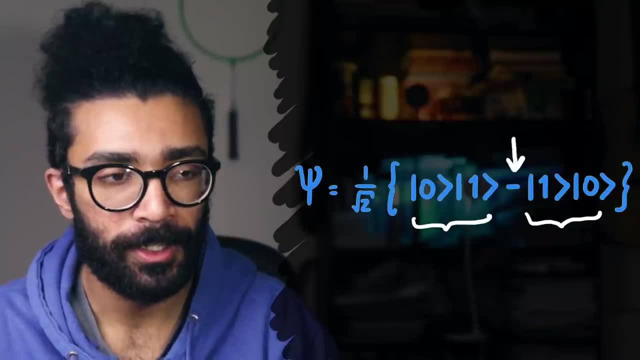 expect from a fermionic anti-symmetric wave function, But, importantly, notice the fact that the two particles cannot be in the same wave function. This is what we expect from a fermionic anti-symmetric wave function, But, importantly, notice the fact that the two particles cannot be. 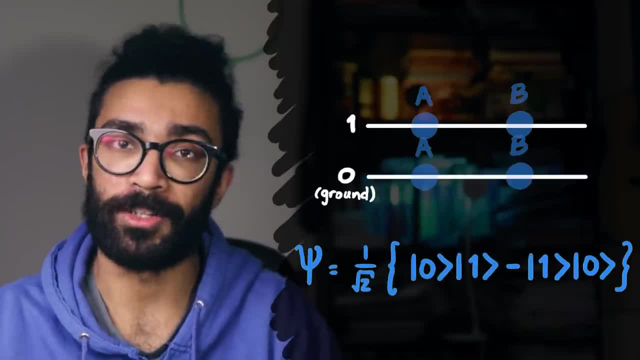 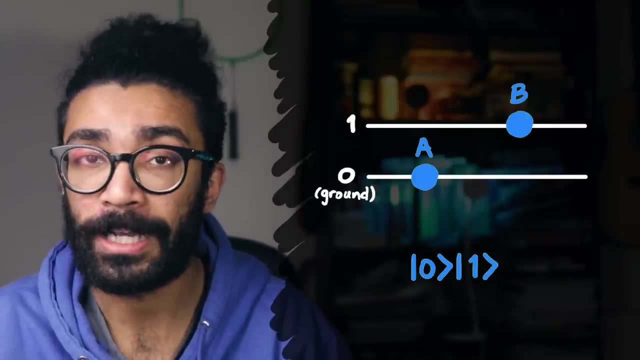 in the same state In this wave function. when we make a measurement on our system, either we'll find particle A in energy level zero and B in energy level one, or we'll find particle A in energy level one and B in energy level zero. This is different to what 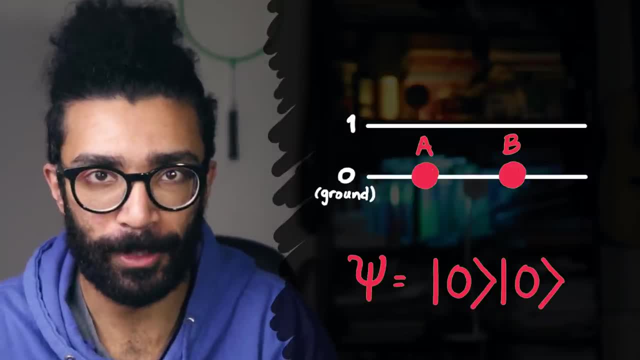 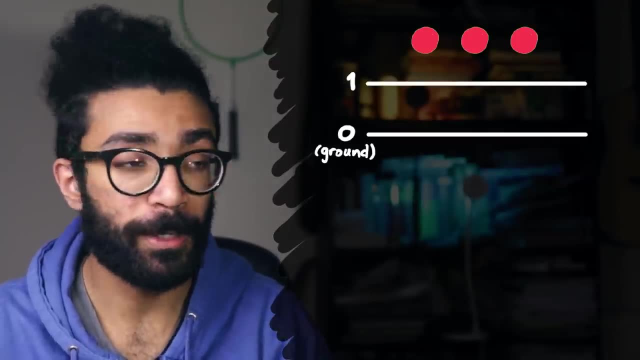 we saw earlier, with our system of two bosons, They could be in the same energy level, And this is a really important difference between bosons and fermions. We can extend this logic to a multi-boson system and a multi-fermion system, and all of these bosons can basically 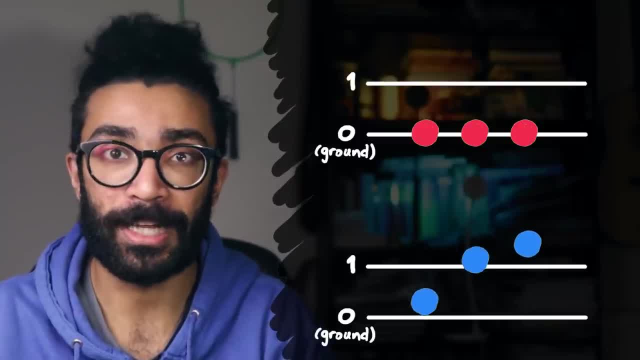 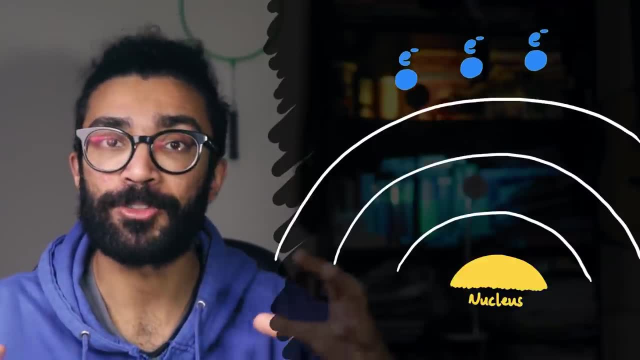 collapse down into one energy level, Whereas fermions cannot do that. they must occupy different energy levels. An example of this fermionic behaviour is the electron shells around atoms. Electrons don't all collapse down into the lowest available energy level, or, for that matter, 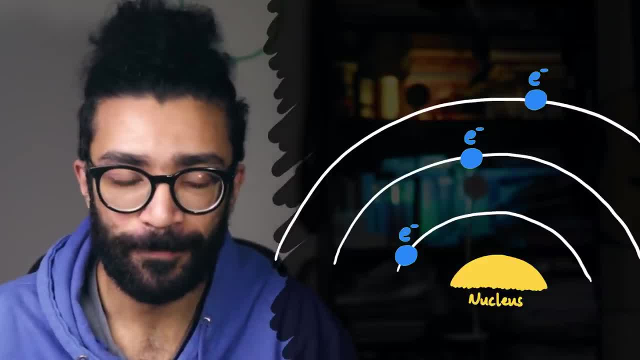 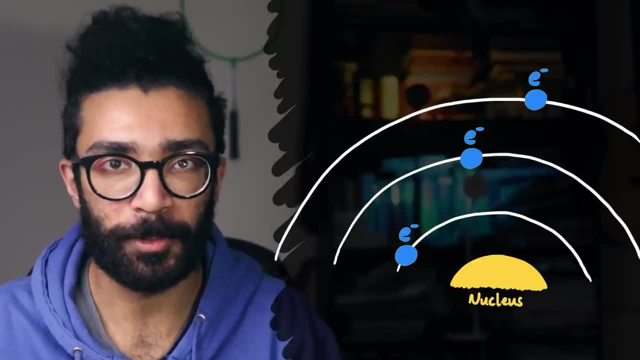 into any one of those energy levels. Electrons are fermions and we see that as the number of electrons around our atomic nucleus increases, the electrons have to occupy higher and higher energy levels, because the lower ones are fully occupied. Now, of course, i've avoided the small matter of spin. 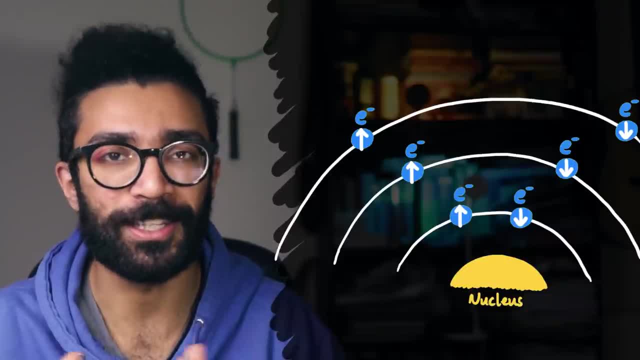 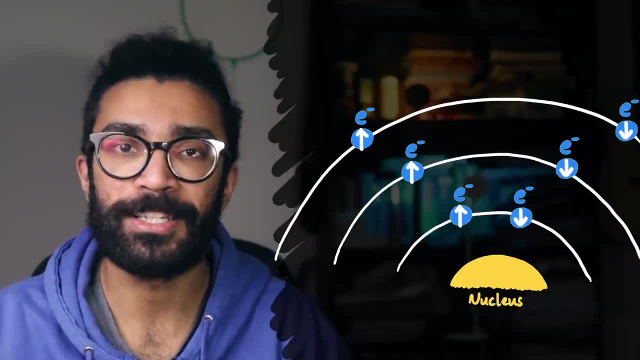 which is actually what allows two electrons of opposite spins to be in the same energy level rather than just one, which is what our basic mathematics was predicting. But that's a slightly different issue, and i want to continue this in a video about the Pauli exclusion principle. 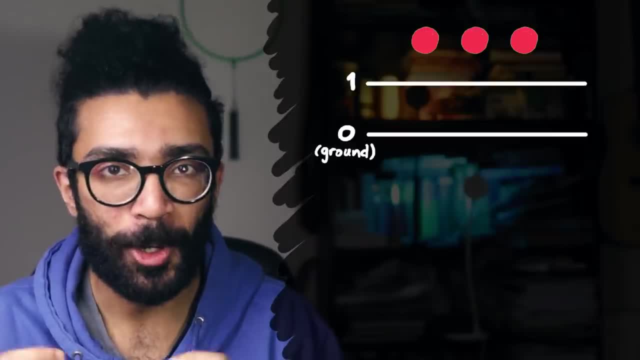 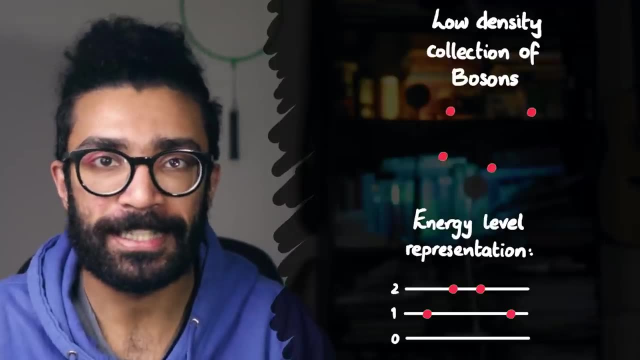 But if we return back to our bosons, then the fact that they can all occupy the same energy level is what allows Bose-Einstein condensation to occur. Usually, when we have a fairly low density gas made up of bosons and we cool it to a sufficiently low temperature, all of these bosons 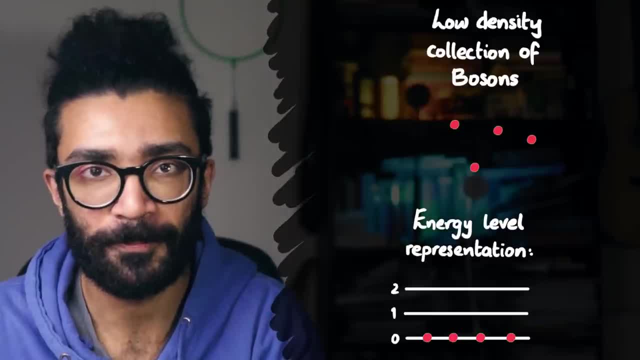 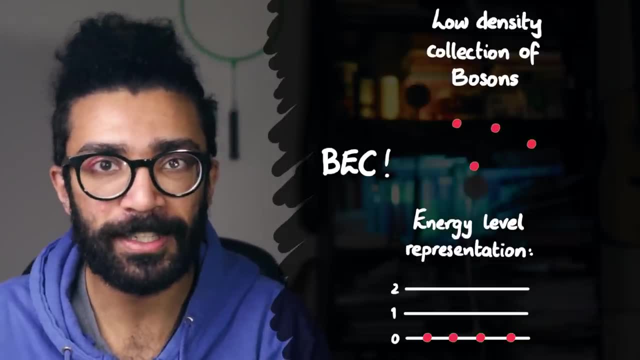 collapse down into one energy level, usually the lowest energy level, And this is a Bose-Einstein condensate. Now the temperature below which our gas of bosons becomes a Bose-Einstein condensate is given by this equation. here Tc is the critical temperature below which we'll have a Bose-Einstein. 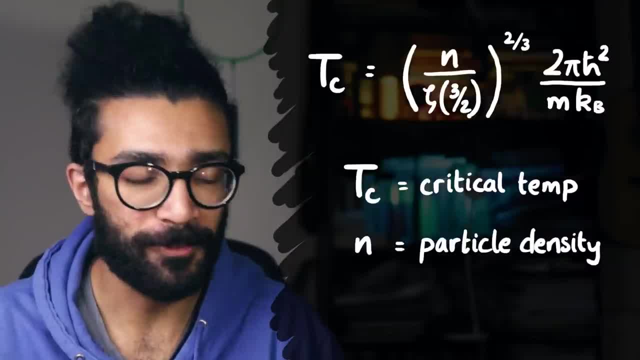 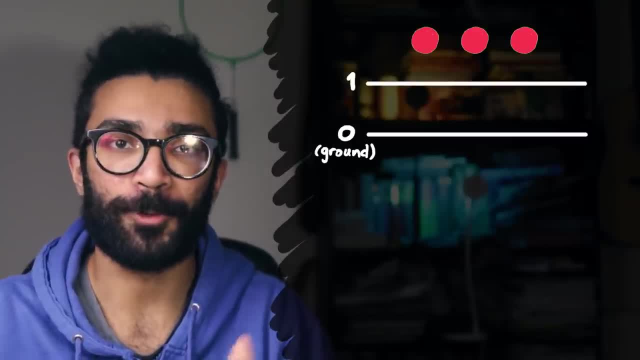 condensate and it depends on a couple of different things like the number, density of the bosons in our boson gas and the mass of the bosons. Now, when we have a Bose-Einstein condensate, when all of these particles fall into the same energy level, we tend to see some rather interesting.